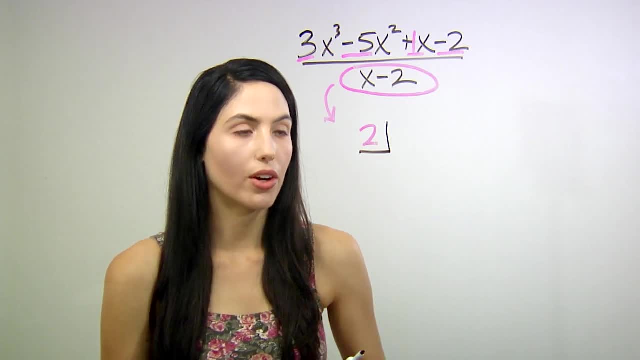 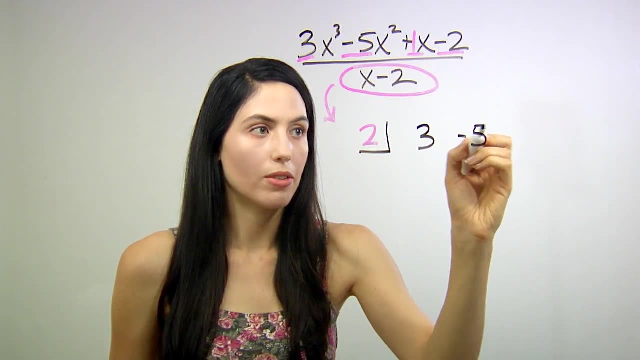 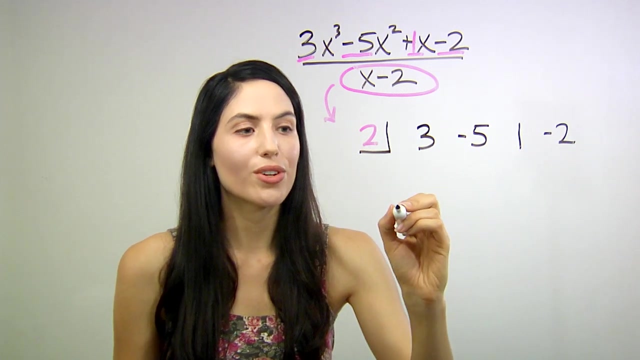 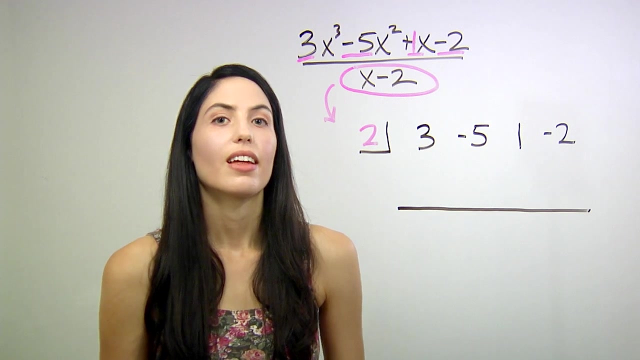 and put them in a row here down below. So we have 3, negative 5, 1, and negative 2.. Next step: draw just a horizontal line here below, leaving one row of space like that. Then we want to drop down this number like that. 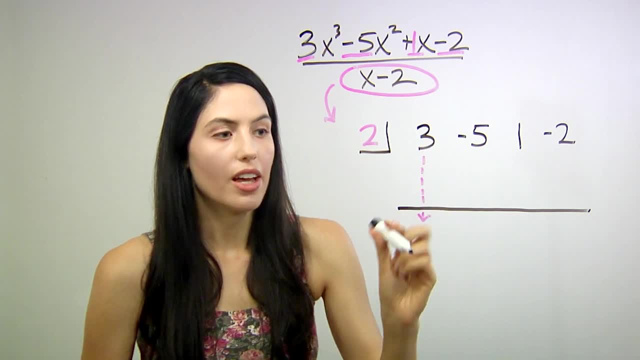 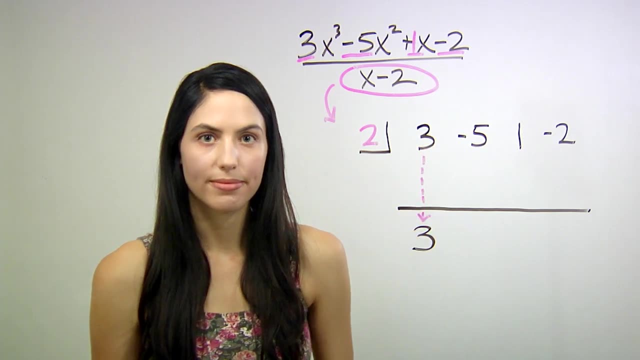 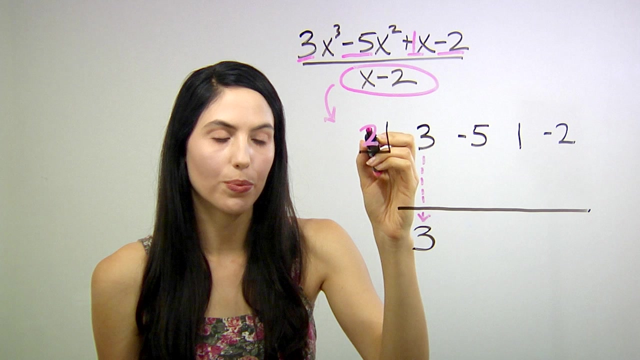 and write it again down here below. So drop down the 3 and write it at the bottom. Next you're going to take that number 3 and multiply it by our constant 2.. So 3 times 2 gives us 6,. 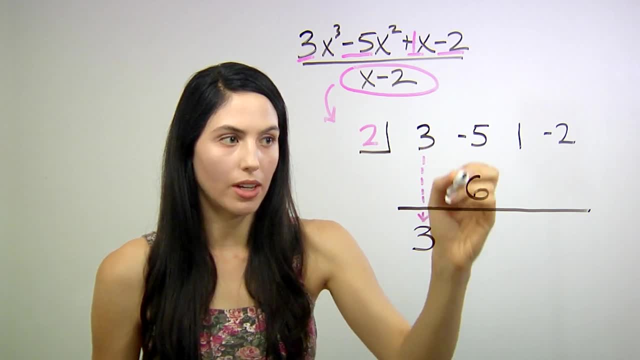 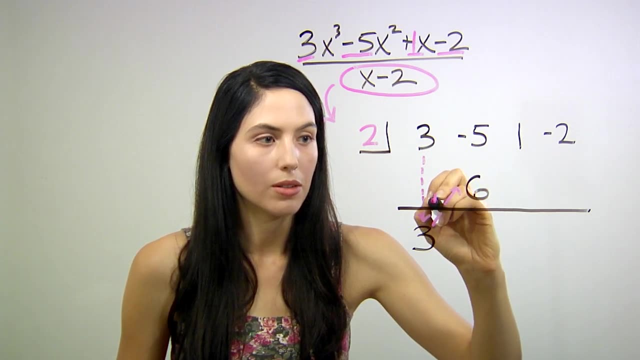 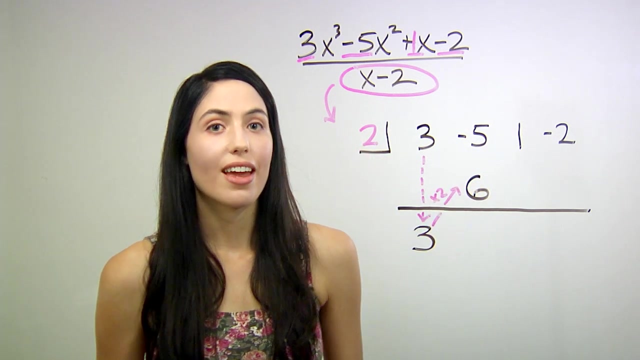 and we write it here in the second row, second column. So that step was: Take your 3, and multiply it by your constant and write the answer here. Okay, then you're just going to add the two numbers in the column. 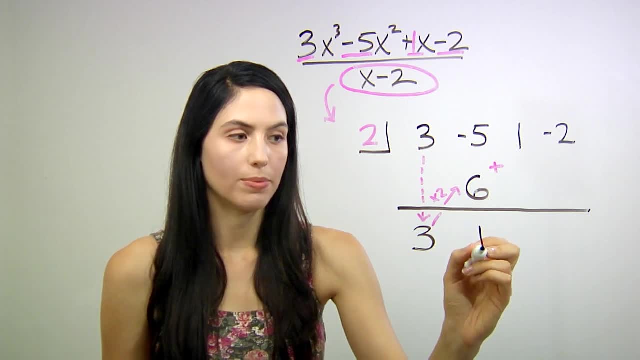 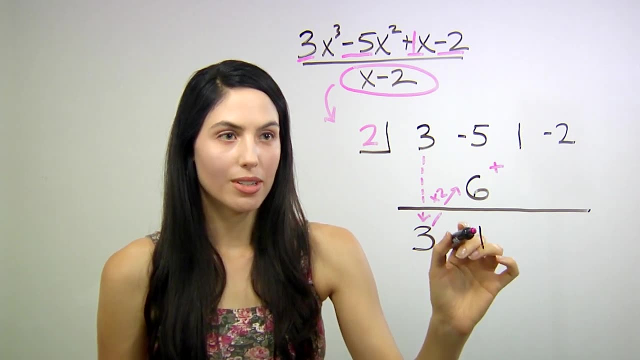 In this case we get negative. 5 plus 6 is positive 1.. Then we're just going to repeat all the steps. So 1, we're going to multiply by our constant 2, and we get 2.. 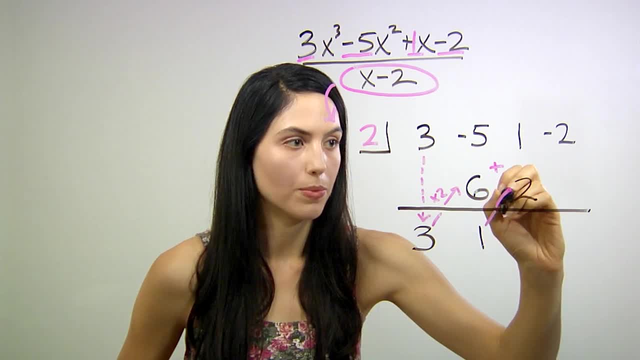 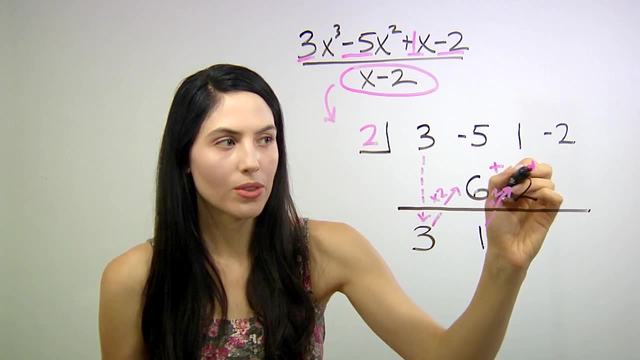 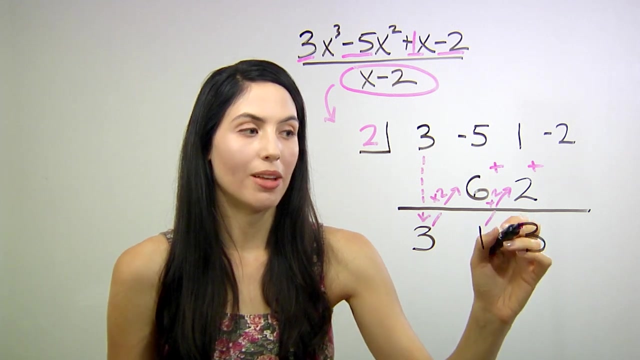 So that step was again multiplied by 2.. Then again we're going to add the two numbers in the column. 1 plus 2 equals 3.. Finally, one more time, multiply our 3 by the constant 2.. 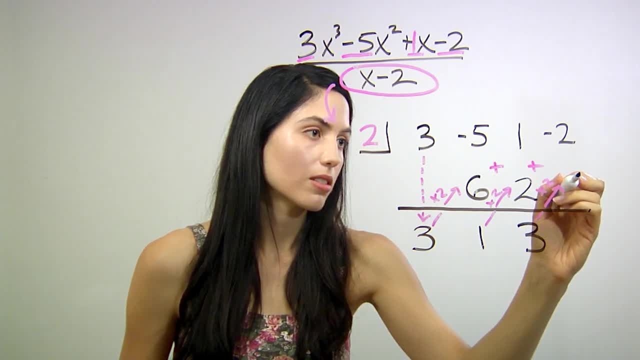 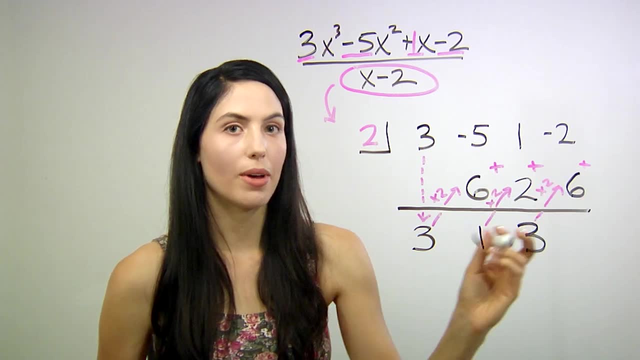 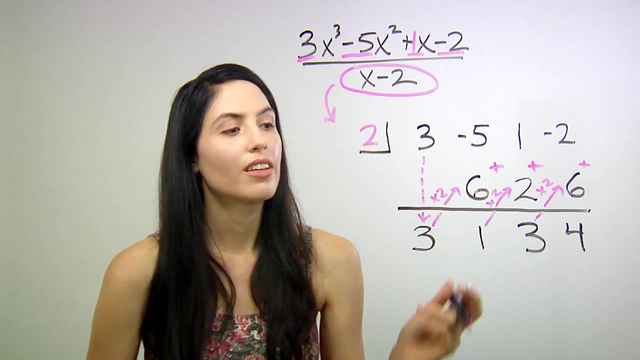 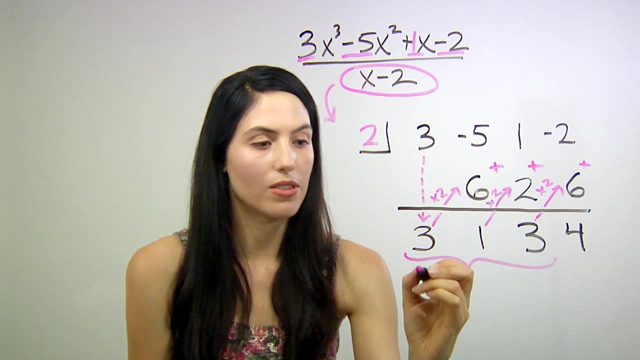 Times 2, we get 6.. And one last time: add the numbers in the column Negative: 2 plus 6 gives us positive 4.. And that's it, Okay, you're done with the division. And these first three numbers are your coefficients of your new polynomial. 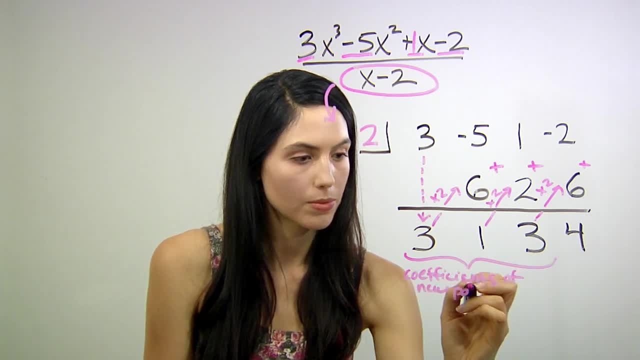 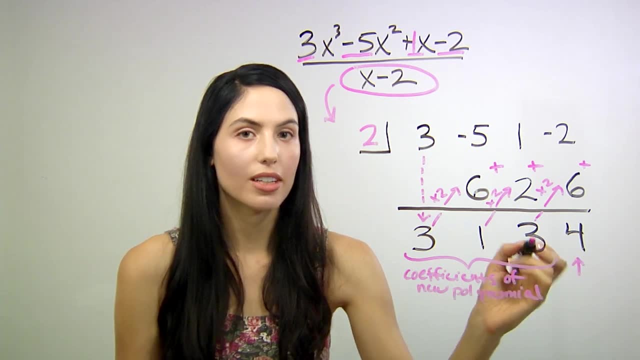 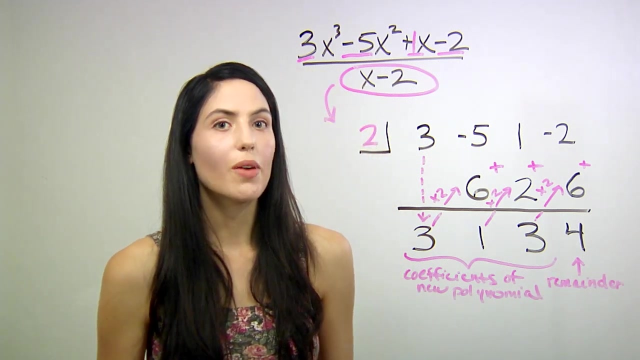 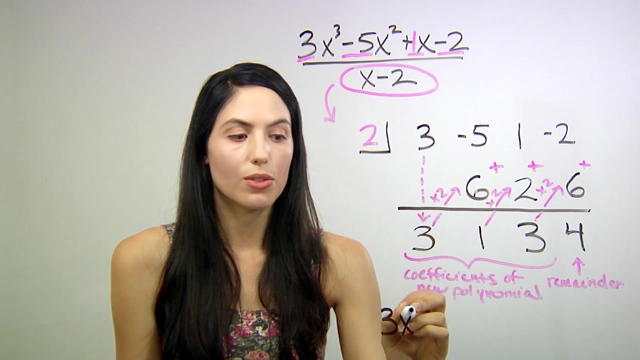 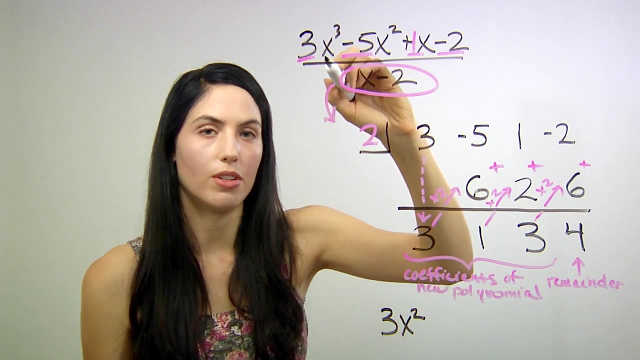 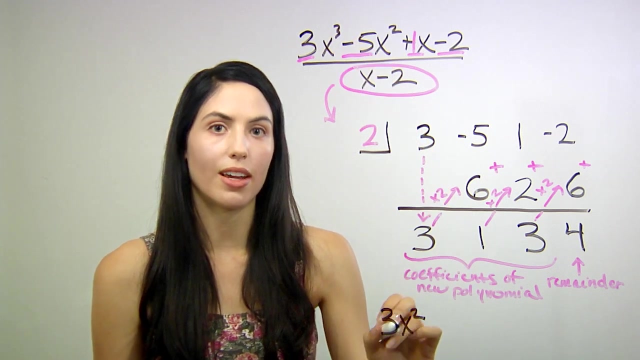 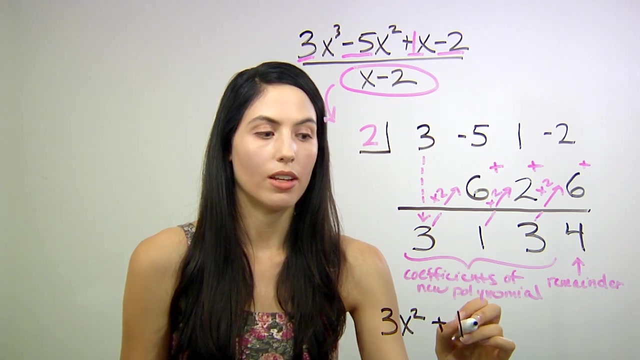 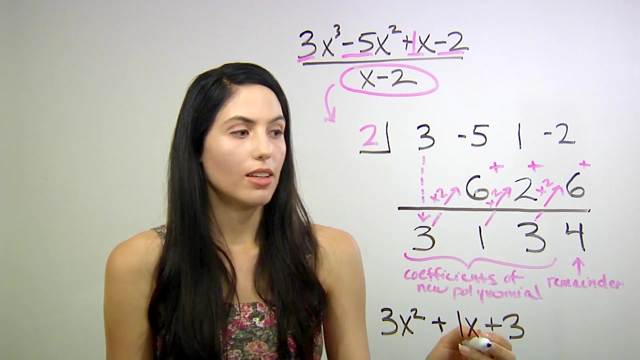 Subtitles by the Amaraorg community. Subtitles by the Amaraorg community. cubed. our answer is going to start with an x squared term. So 3x squared plus one term lower would be 1x, x to the first power plus 3, just a constant. 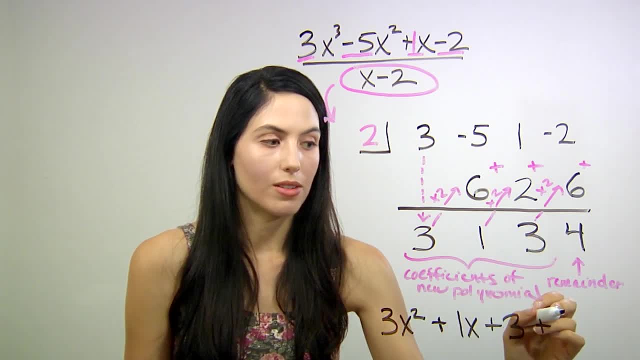 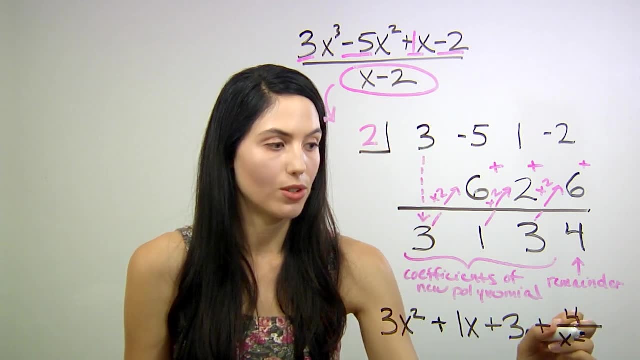 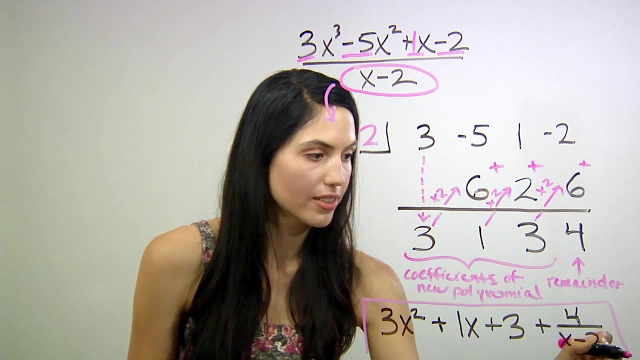 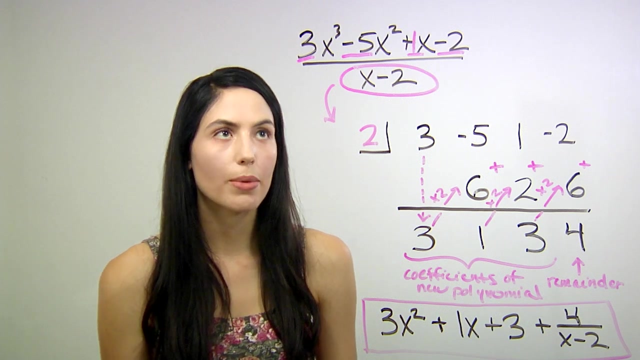 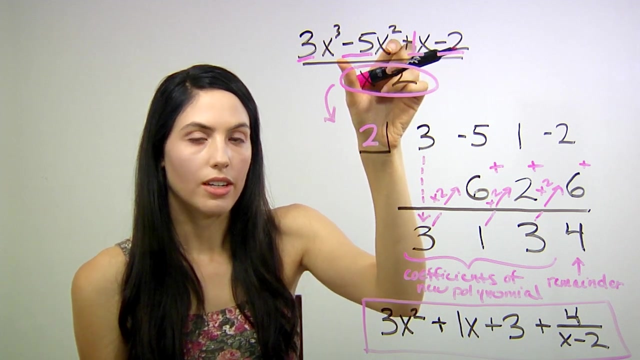 And your remainder you will just write as 4 over your denominator x minus 2.. And that's your answer. So what trips people up is that sometimes you'll get a polynomial where there's a missing term. Say, you didn't have an x squared term here. 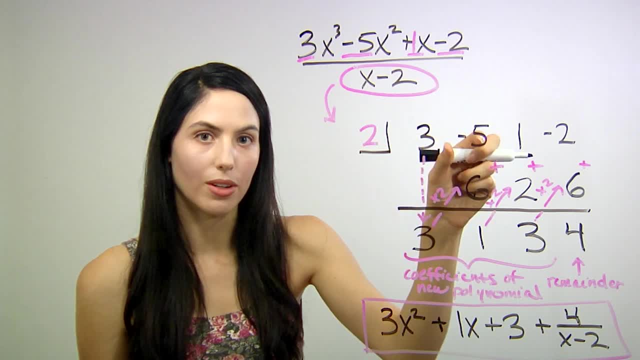 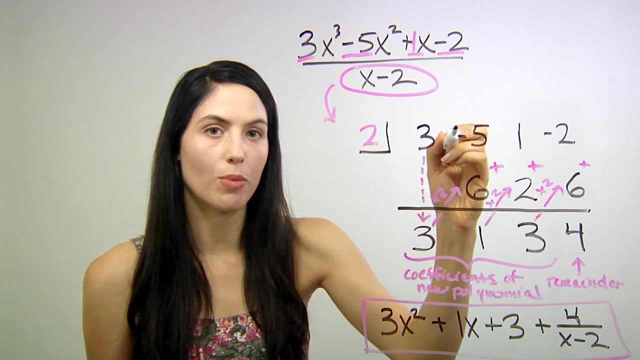 You would actually need to put a 0 term as a placeholder instead. So if there was no x squared term, for instance, you would actually put 0 here. So remember to do that. Another thing to remember is that sometimes you don't have a remainder. 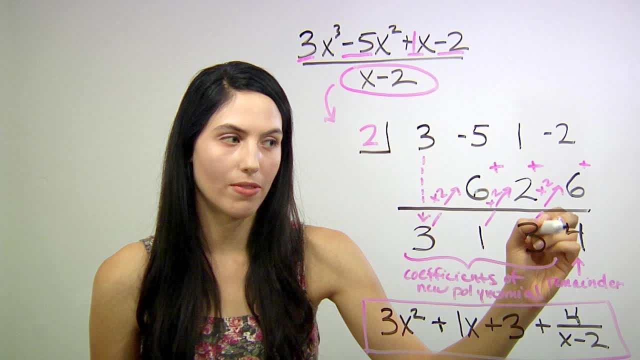 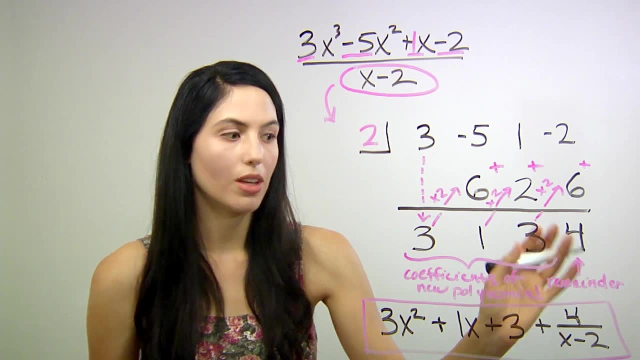 Sometimes you'll get 0 as your last number in the final column of your synthetic division, And that's fine. That just means that you won't have a fraction as your last term. That won't even be there And you'll just have a polynomial. 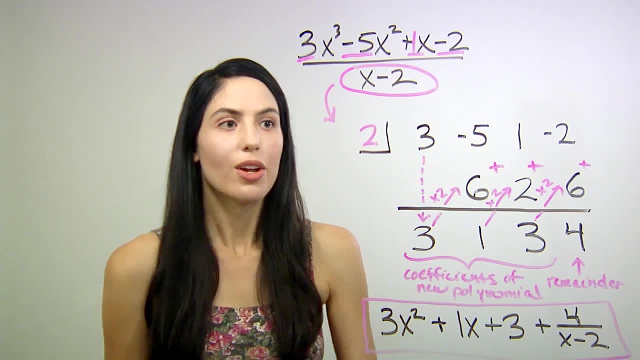 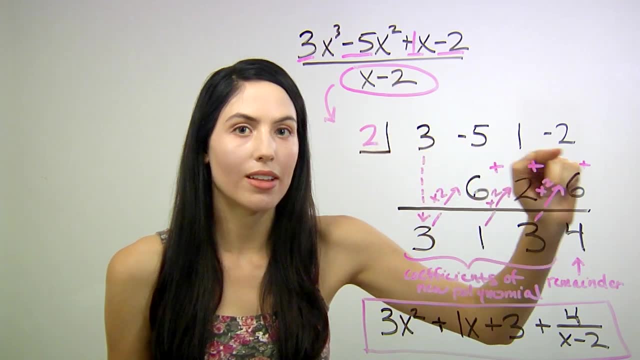 OK. so to summarize, the steps for synthetic division are right here in the corner, the number that makes the bottom of your fraction 0.. Write the coefficients of the polynomial from the top of your fraction. If there's a term missing, put zero instead. 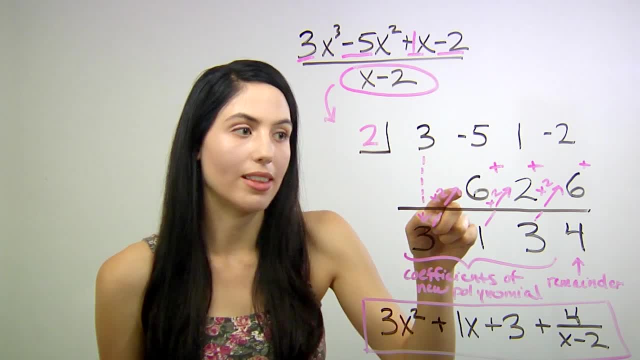 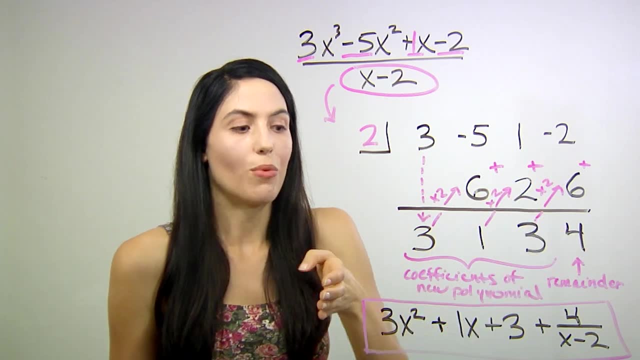 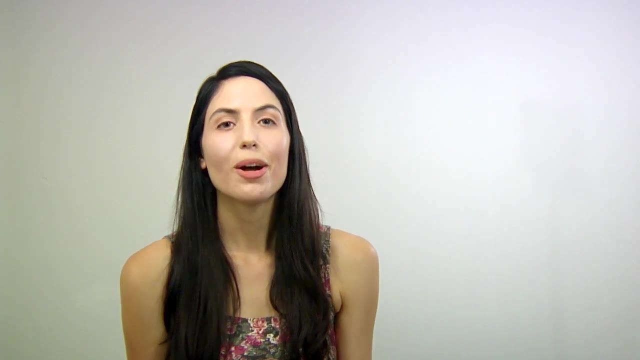 Bring down the first number, multiply it by a constant, write the answer here, Add the column, repeat those steps until you get to the end of your synthetic division and then write your final answer using those numbers. Good luck, I hope this helped you understand.